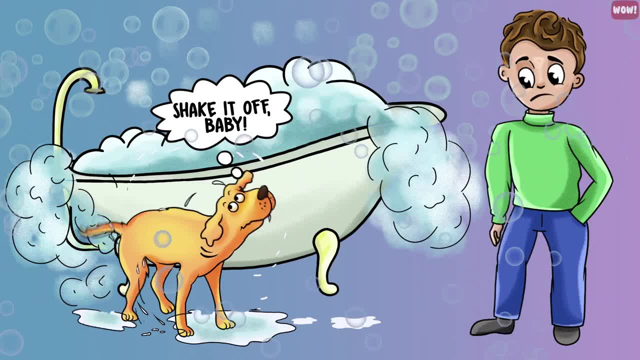 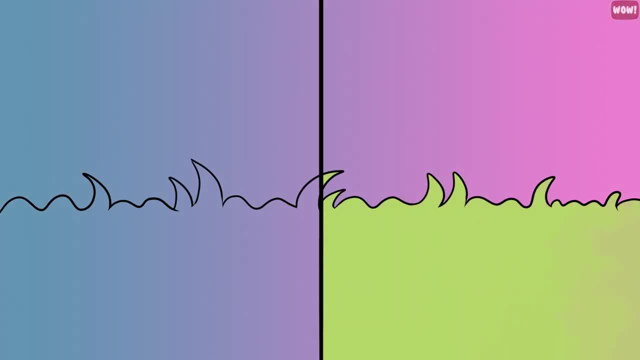 in mind. if dogs get too wet, they will shake off the extra water as an instinct to dry themselves faster. Dogs and cats will also try to please you in the best way they know. A cat will try to impress you by killing a real mouse and bringing it to you as a gift. 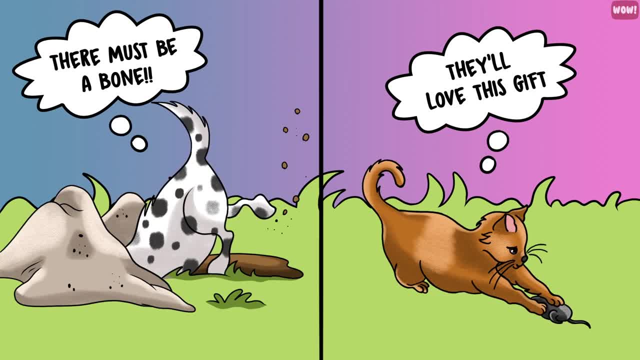 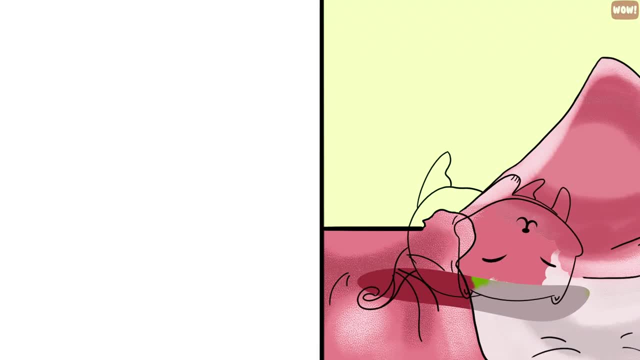 At the same time, a dog will dig holes in the yard to bury bones for future nourishment. They will also chase squirrels away to protect your property. Now let's talk about how your pets spend the day when you are at work. Cats spend. 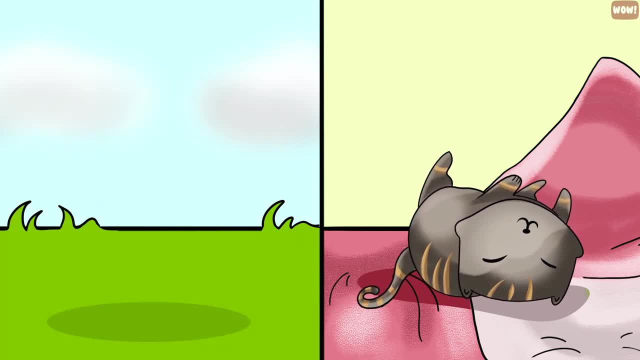 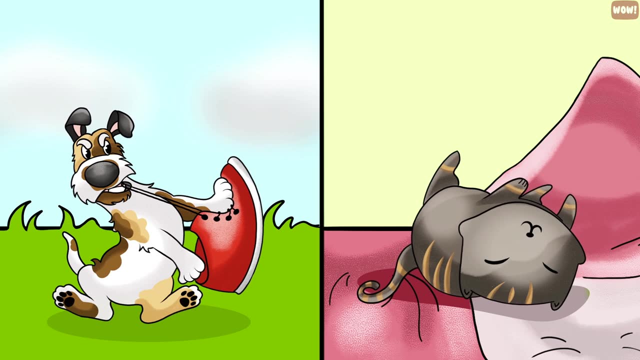 about 75% of their time sleeping during the day. On the other hand, you may find that your dog has chewed up a pair of shoes. They do it because your shoes have your scent on them. Your dog chews on your shoes because it not only relieves 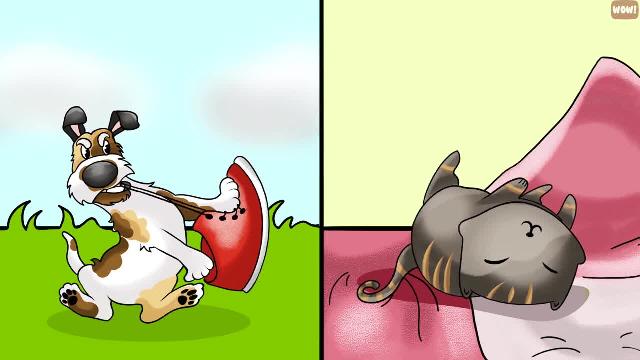 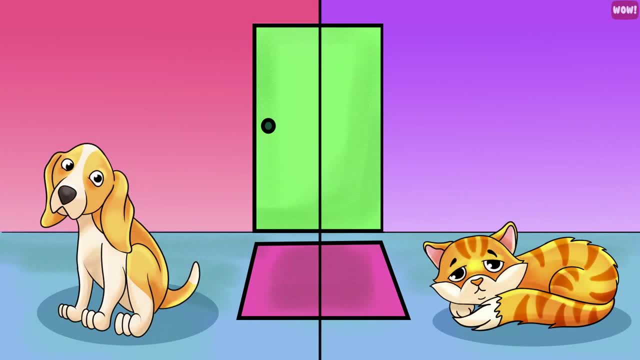 their stress, but also releases endorphins that make them feel better when you're not at home. They may also tear up furnitures And keep in mind. your dogs and cats don't know when you are coming home, so they can become anxiety-ridden just like anyone else. 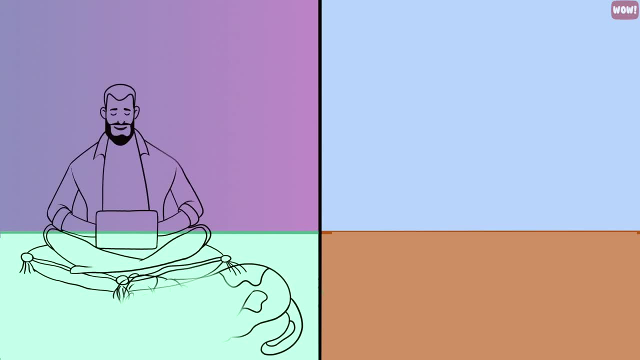 It's the same reason. a cat purrs when they jump on your lap or on your laptop. So while a dog is a little more respectful of your space when you are working at home, a cat might just jump up and sit on your lap. 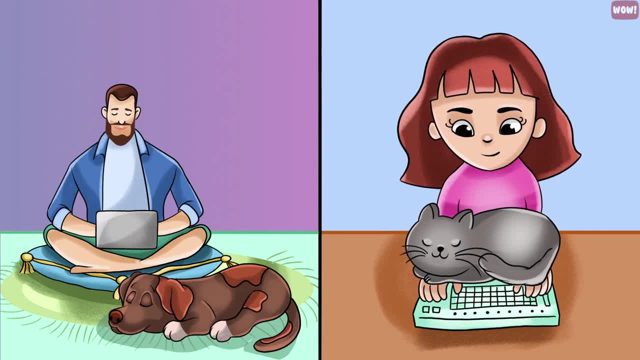 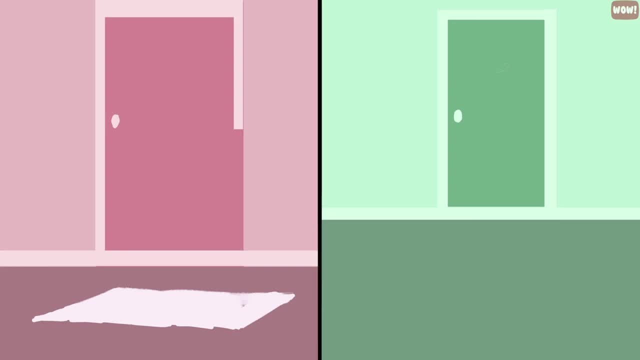 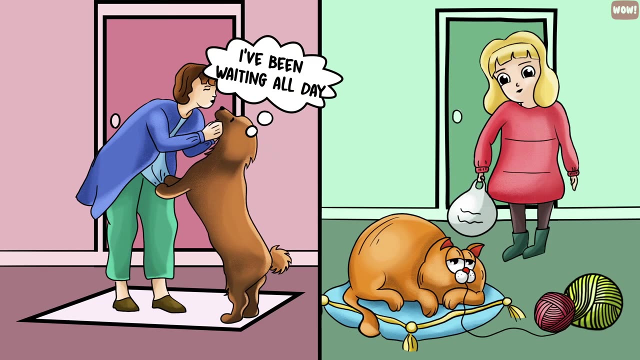 That is when they feel like it. Now let's talk about how dogs and cats greet you when you come home. While both pets have a sensitive sense of hearing and a profound sense of smell, cats and dogs are very different creatures. So, while a dog will jump up to greet you because they are glad to see you, 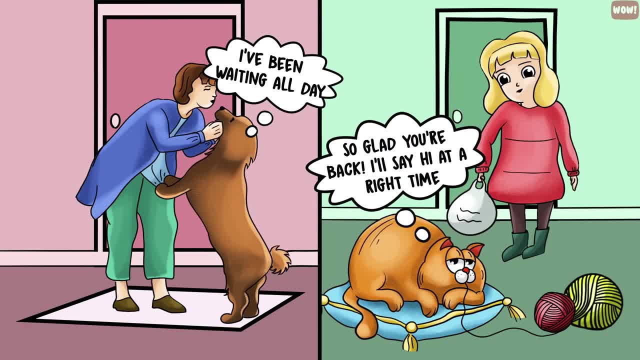 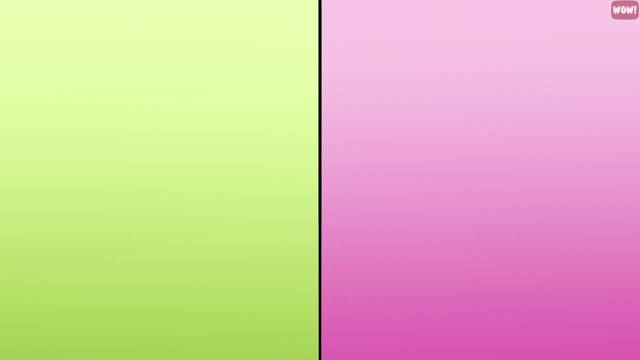 at home. a cat is a little more standoffish. They'll greet you or any of your guests when they get in the right mood. Speaking of the weekend, this is also playtime for cats and dogs, And while you can take your dog outside to chase a ball, your cat may play on its own. You can even buy a cat. 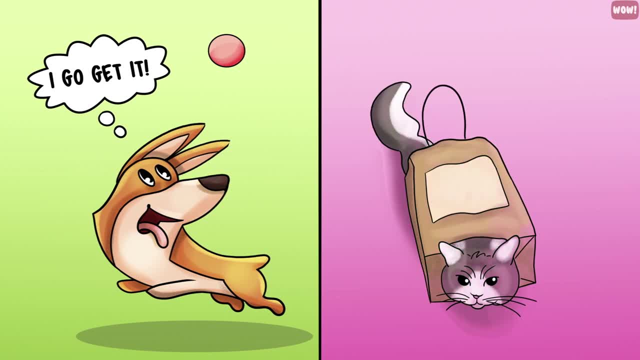 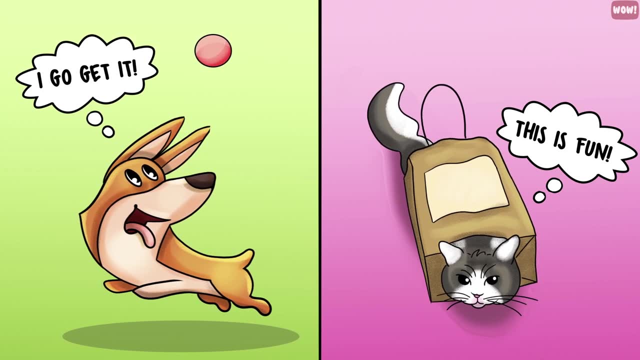 an expensive toy, but cats are more likely to play with a small stuffed mouse or a paper bag that is left on the floor. So while dogs are interactive with their owners, it may be more fun to sit back and watch the fun when a cat finds the most unlikely entertainment you can think of.